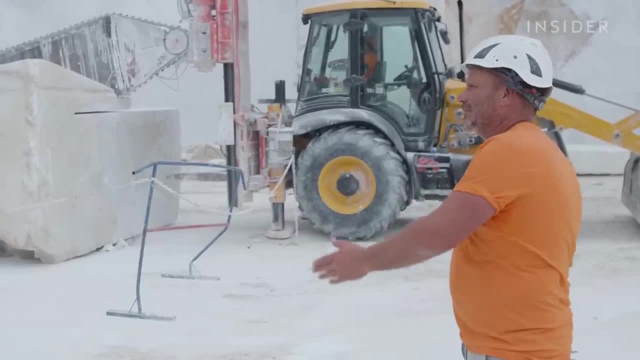 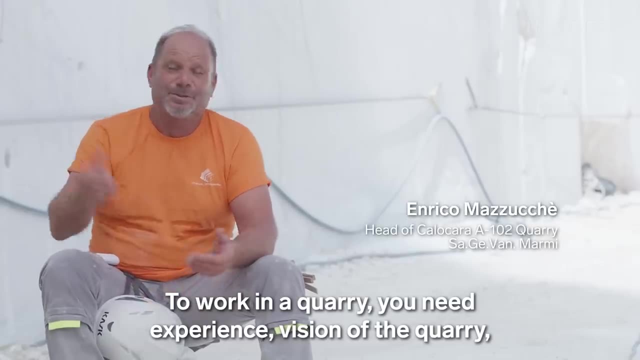 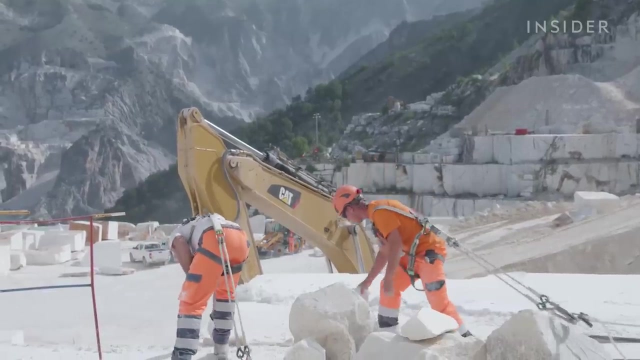 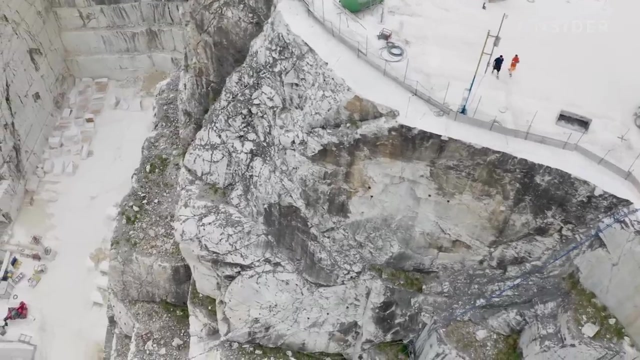 Enrico has been a miner for 40 years. He learned from his father, who worked at the same quarry. It's important that miners have a trained eye and are precise. They need to work around the mountains' defects to avoid the risk of the marble breaking. 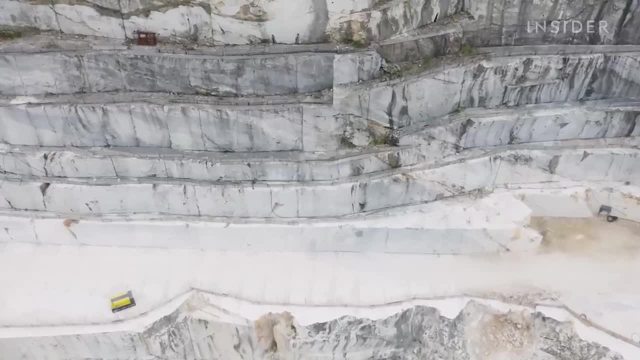 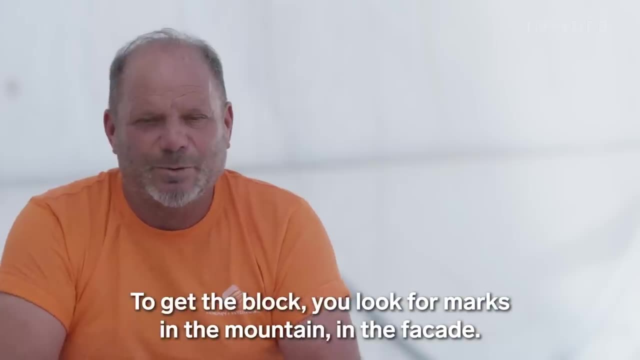 These flaws affect where the miners can extract, how much they can extract and, eventually, how much they can sell. To cut the block, to pull out the block. we look for signs in the mountain, in the bank, in the front. 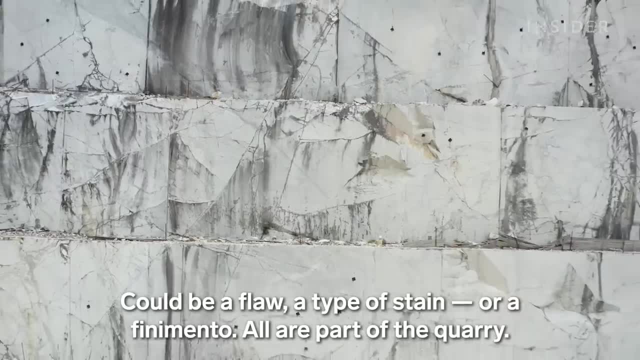 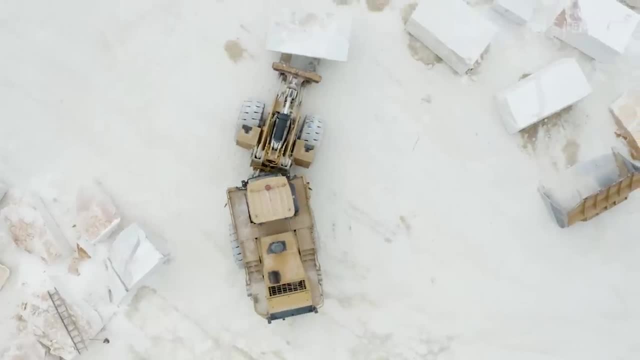 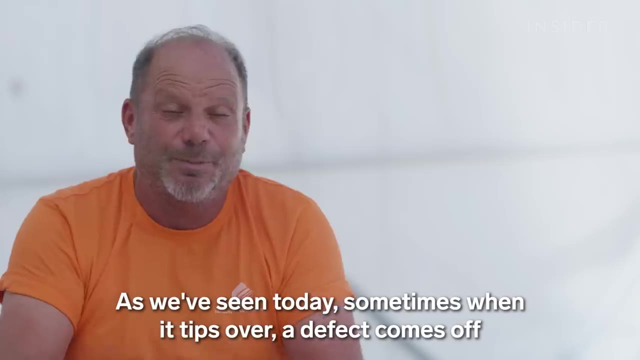 A defect, a kind of stain, a finish- These are all things that are part of the cave. Despite Enrico's care and attention, he doesn't always get the result he wants, As we've seen before when the block is turned over. 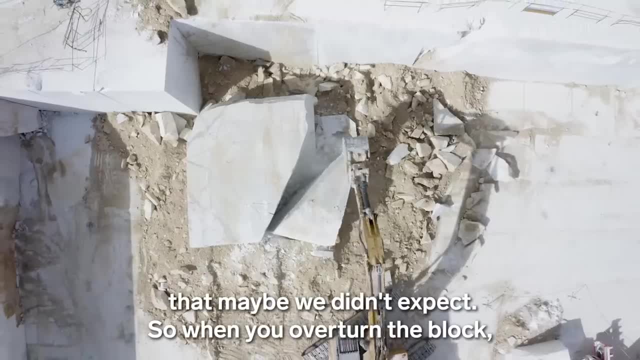 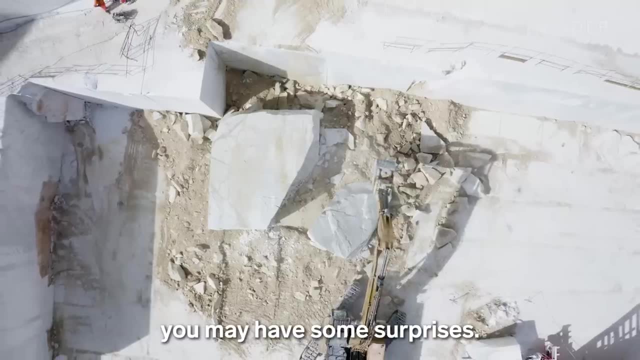 a defect is removed. that was expected, but it can also be from behind that you didn't see. So when the bank is turned over, the criticality can be that. But before they can detach the block they have to drill and saw. 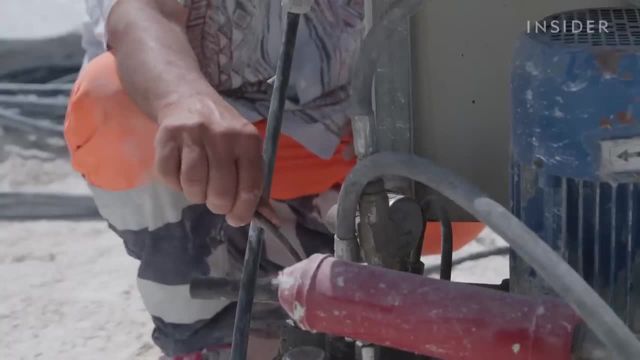 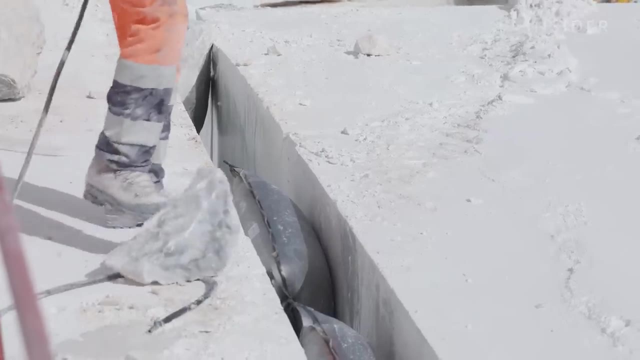 In the first stage of extraction, miners use drills to make strategic holes in the mountain. They then run diamond braid cords through these holes, cutting the marble into a block. The machinery is kept wet to protect the marble, as chainsaws help detach the block from the mountain. 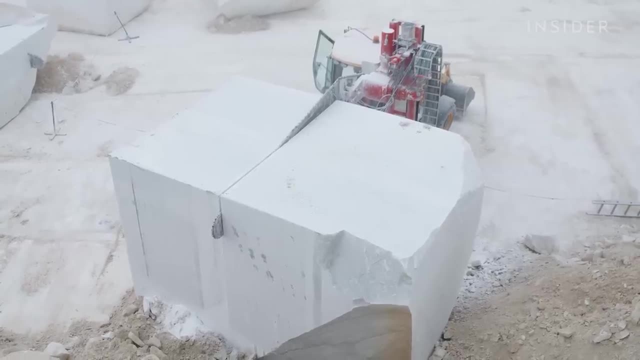 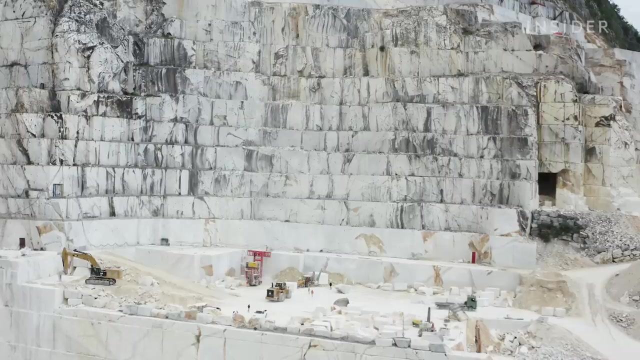 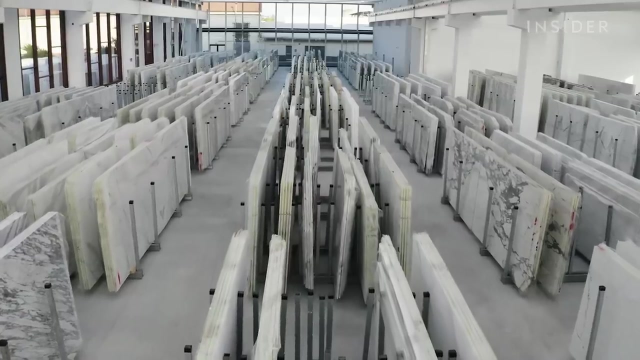 An average block is 12 cubic meters and can weigh 36 metric tons. It's then carefully loaded into a truck, which brings it to a processing facility. Here the Calacutta marble blocks are sliced into slabs. At this stage, processors can't afford to make a mistake. 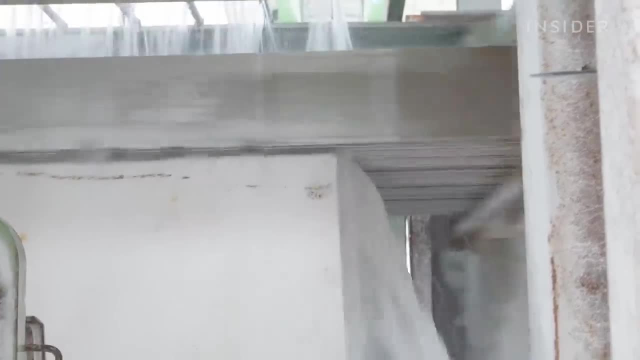 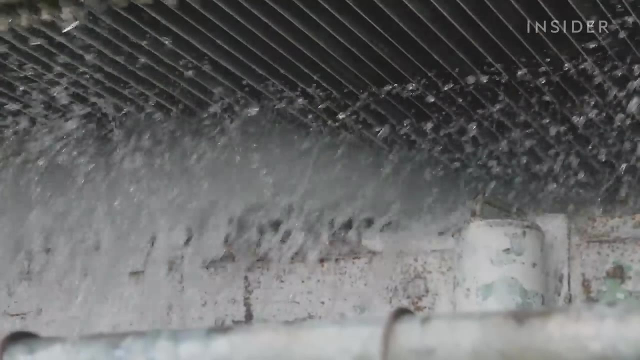 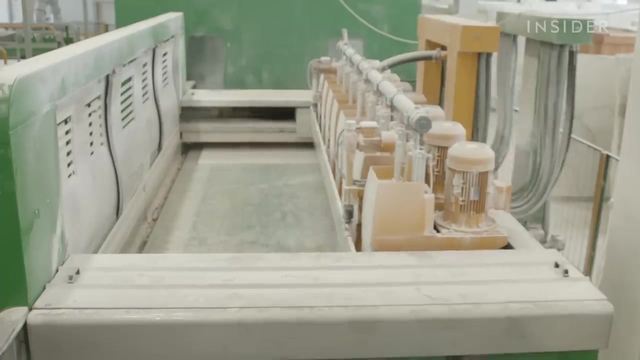 and risk ruining the rare marble delivered to them. They mount over 100 very thin blades onto a wet saw and the cutting begins. The saw cuts slabs as thin as 2 centimeters. Then they're prepared for shaping and polishing. The slabs are first sanded and pre-smoothed. 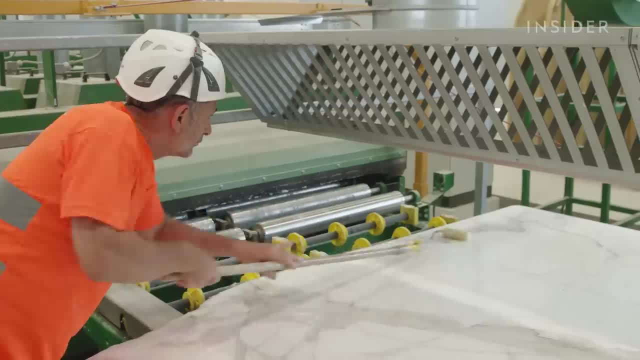 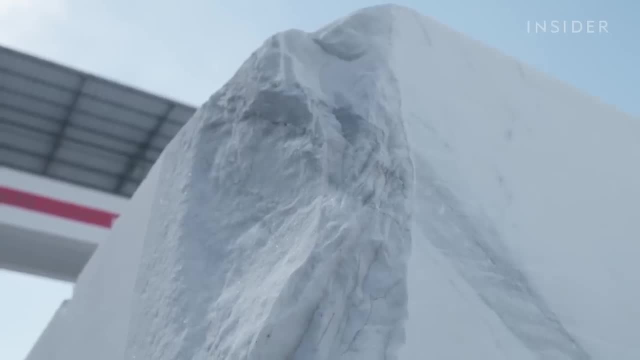 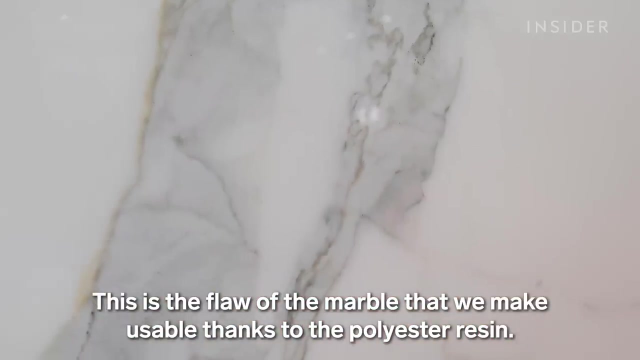 Then they're prepared for resination or the application of resin to fill any cracks or holes in the slab. It's also used to attach broken pieces like the ones that cracked at the quarry And with marble as rare as Calacutta. 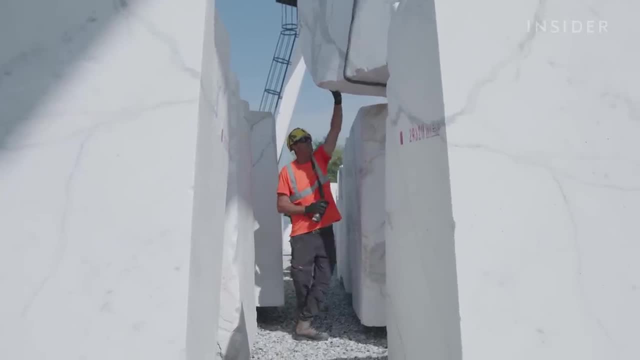 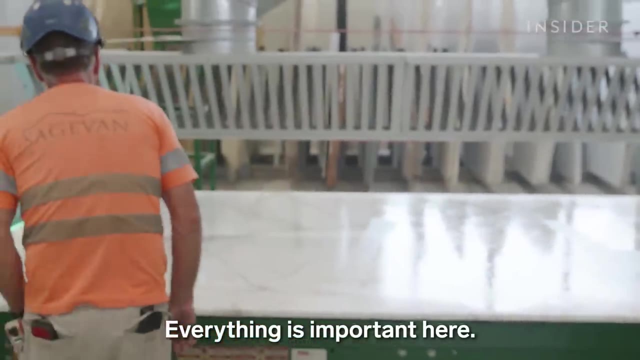 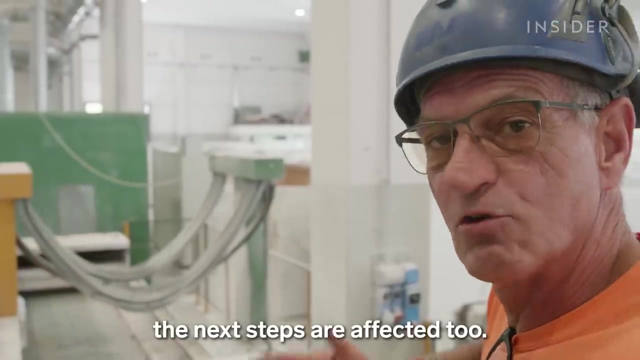 one mistake can have a big impact on the quality and final price of the slab. It's not done correctly. Later, the various stages are not done correctly, So we have to start right away from the first stage to do it correctly. 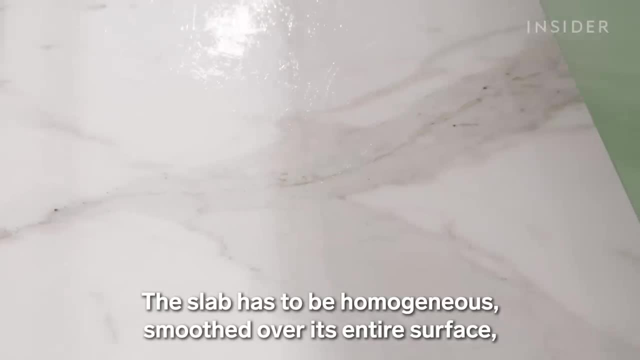 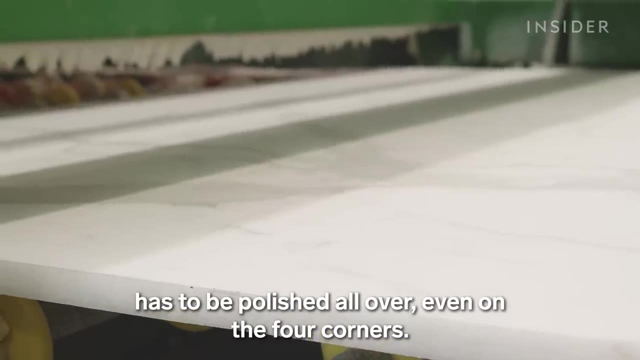 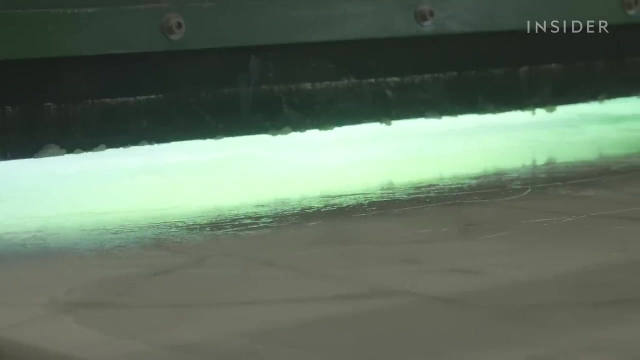 So the slab has to be homogeneous: slanted over its entire surface, over the entire width of the slab, also over the various four corners. After Sergio checks that the resin was applied evenly, he moves it under UV light to dry. These steps ensure that the slab has no flaws. 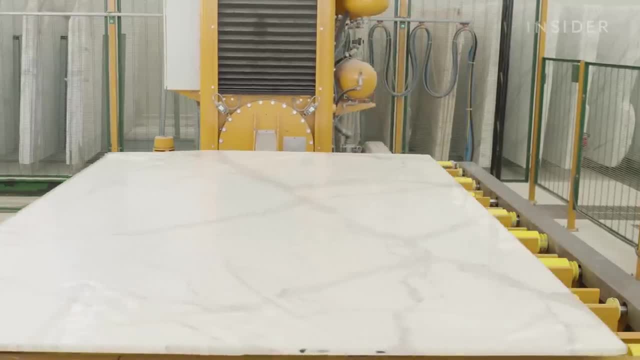 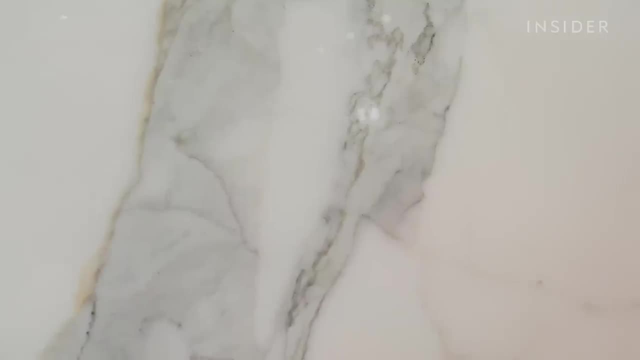 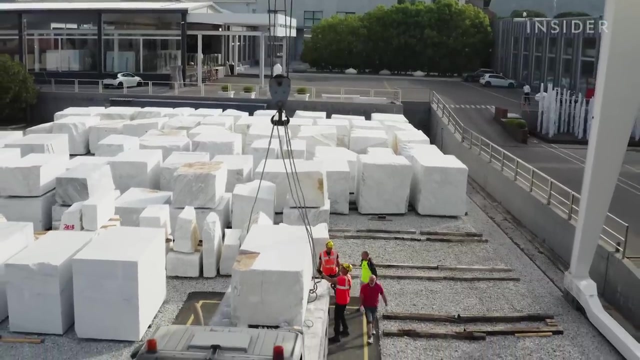 Then the Calacutta slab reaches its final stage. It's honed and polished until it almost sparkles, becoming, as Sergio says, shiny to the eye. It's now ready to be sent to the buyer. Calacutta is extracted and processed on a per-order basis. 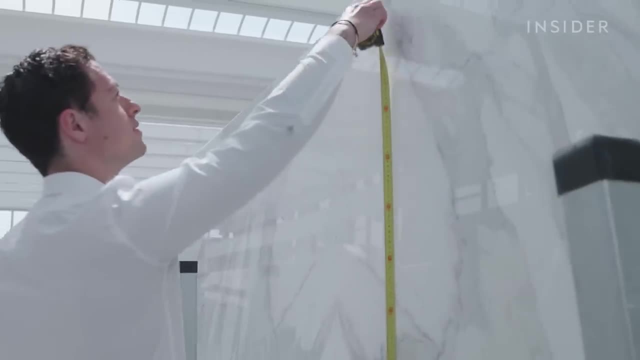 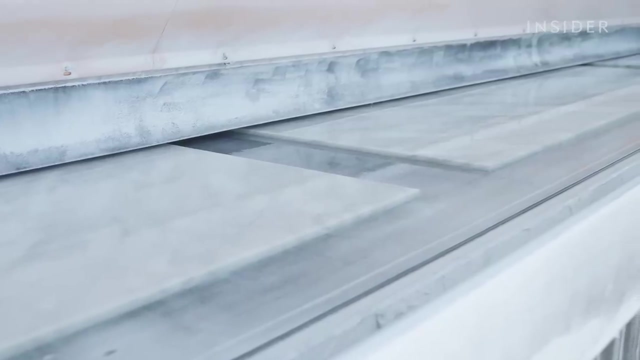 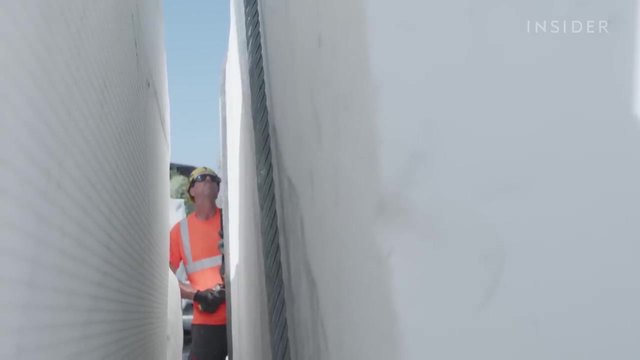 Producers consult the customer every step of the way. This way, the Calacutta is perfectly customized to the client's needs, because once it's fully processed, there's no going back. Even with these risks and high costs, customers still want Calacutta. 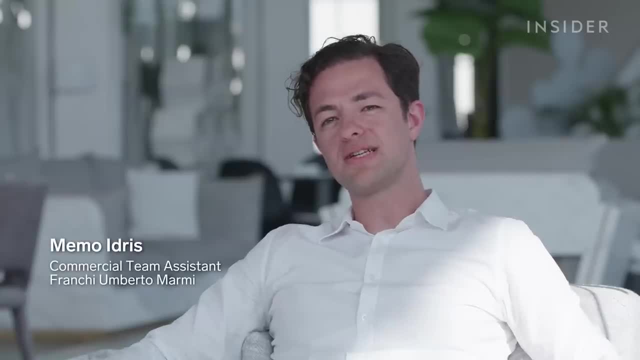 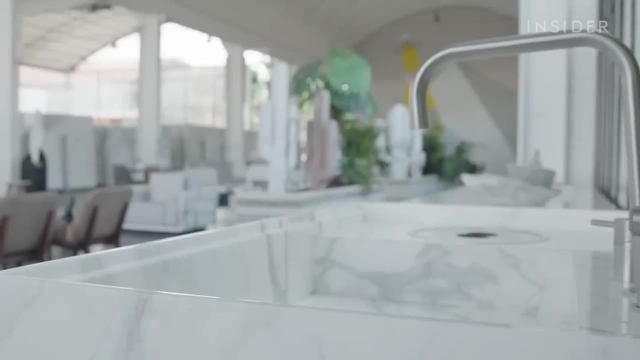 Our customers prefer Calacutta because it's a luxury, it's a high-end product, it's timeless and it's classical. It fits very well with any kind of furniture. White marbles like Calacutta are more desirable because they have fewer flaws than darker marbles. 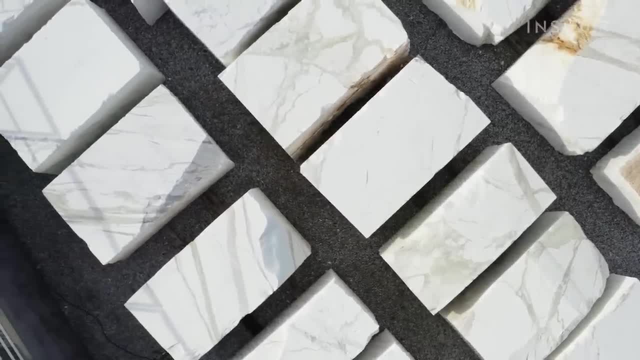 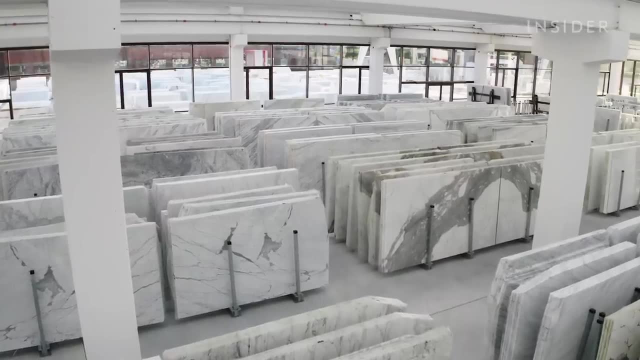 so they require less maintenance and repairs. Calacutta is in even higher demand than other white marbles like Carrara. The veins look crisper, less faded. There are generally fewer veins in Calacutta, making it easier to incorporate in exterior and interior design.